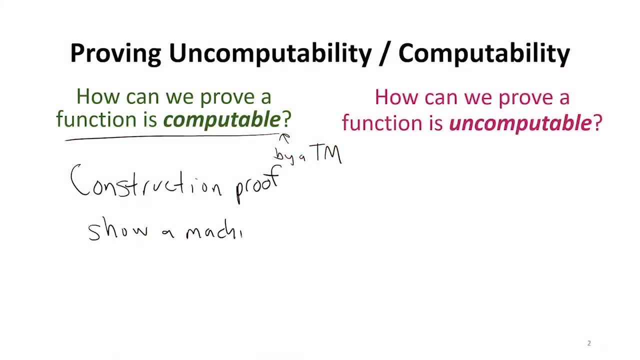 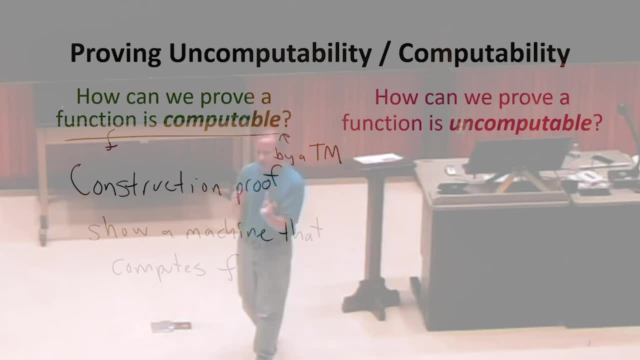 is: construct some machine that computes, let's say, a function f. And what does it mean to have a machine that computes it? It's a machine that computes a function f. And what does it mean to have a machine that computes it? Well, it has to, for all possible inputs, produce the correct. 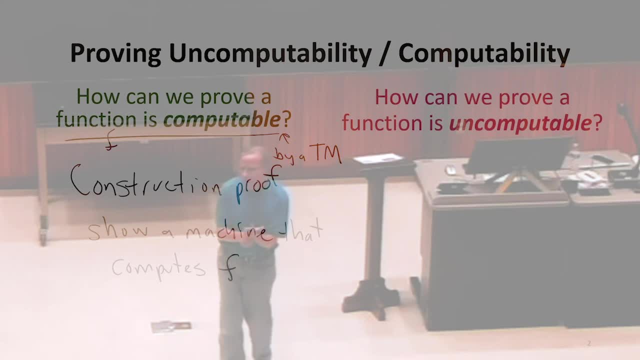 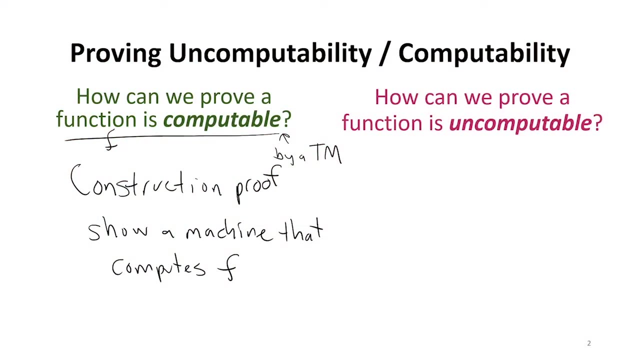 answer, And that means it always finishes and it always produces the right answer. Yeah, question, Good question, yeah. So what does it mean to do a construction proof? So if our goal is to show a Turing machine, would it be enough to show a Python program? What would make you really convinced? 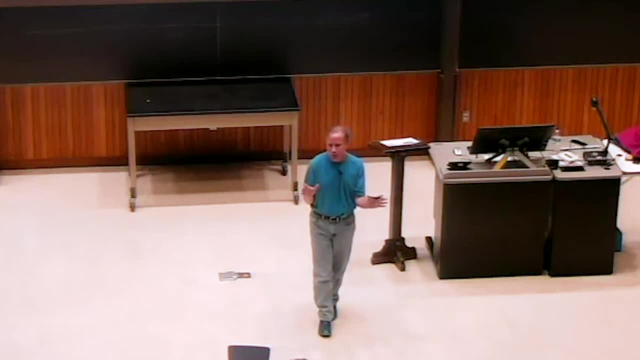 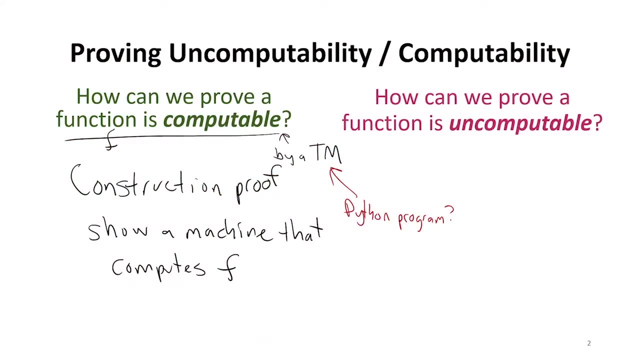 that the answer- if you show a function, show Python code that computes it- that that's a satisfactory answer to prove something is computable by a Turing machine. Yeah, So how do we know that? How do we know that anything we can construct in a Python program? 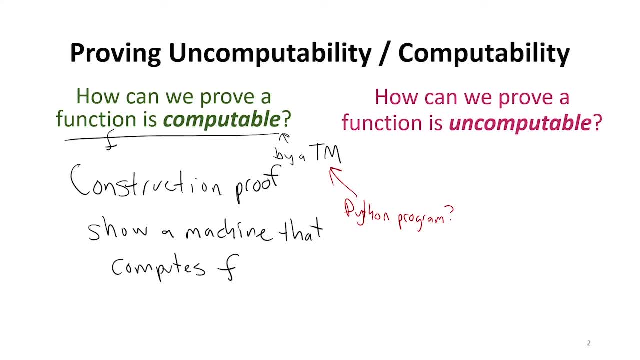 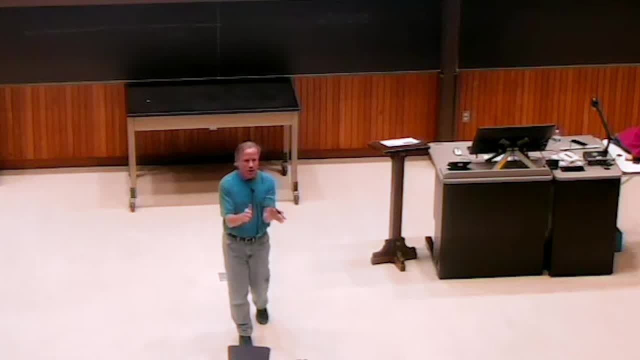 we could also write in the Turing machine To show that something is computable by a Turing machine. if we're going to do it by writing something else, we've got to show that whatever we did that something else in, we can simulate with the Turing machine. 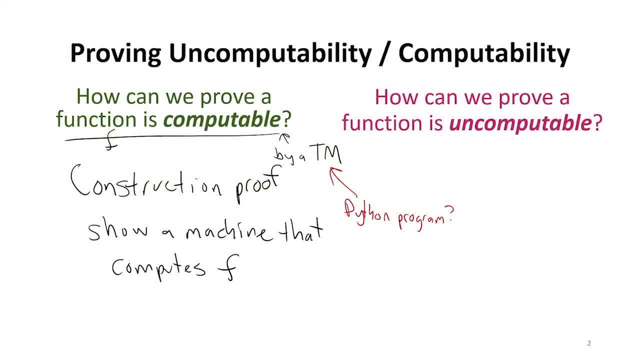 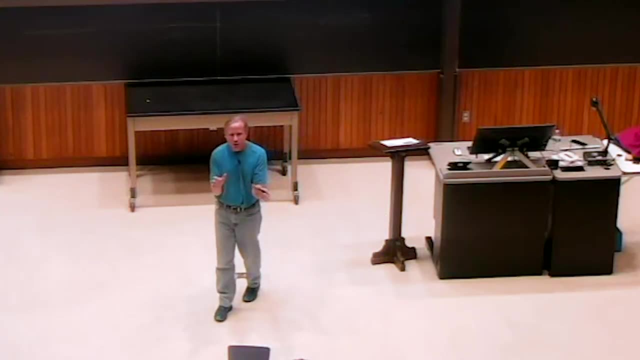 So if we can write a Python program and we can show that there is a Turing machine that simulates Python, so once we've shown that there's a Turing machine that can simulate Python, anything that we can do in Python we can also do with a Turing machine, because we can simulate. 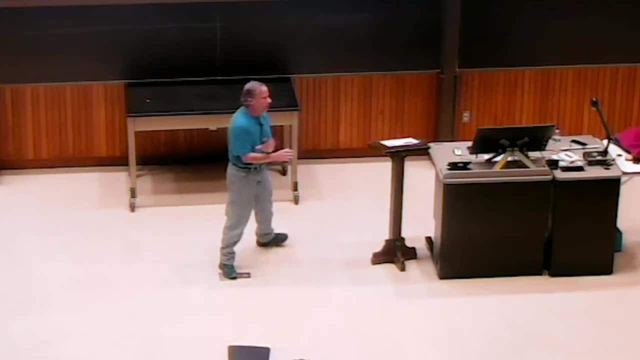 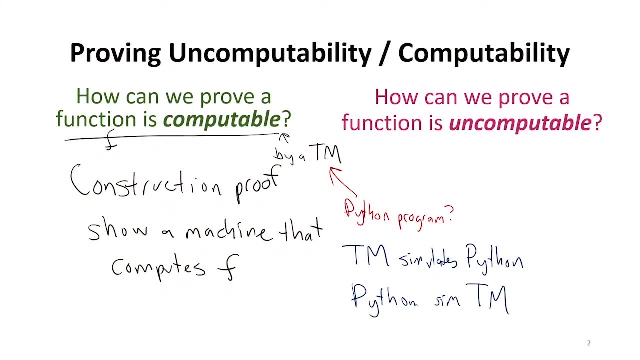 Python with that Turing machine. If we wanted to show the opposite, we'd have to show. if we could show writing a Python program that simulates a Turing machine, that would mean anything that we can do with a Turing machine, we can also do with Python, At least in our idealized version of Python. 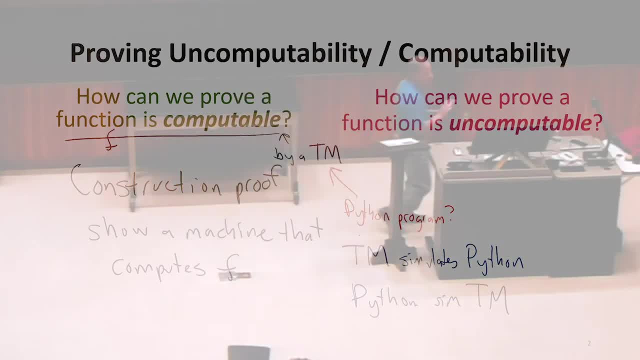 we could do both right. That would show that they're equivalent. But if our goal is to show something is computable, we just need the one direction. If your goal is to show something is computable and you say: well, I know that I can write a Turing machine that simulates Python. 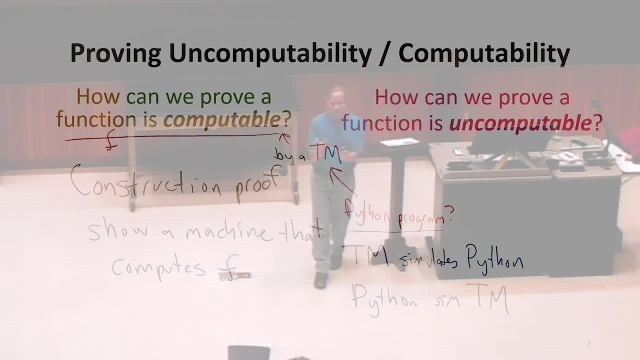 then I can show my computability proof by writing a Python program, because I know that there's a Turing machine that would simulate that It's easier to write Python code than to write Turing machine code. That's the usual way we're going to prove something is computable is by construction. 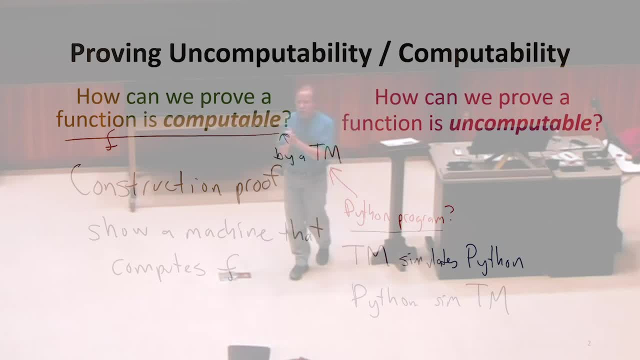 by showing a way to compute it. And that doesn't necessarily mean we know the specific code or we know the specific Turing machine description, but we know that there's a way to make it. So what about proving something is uncomputable? If we're going to prove uncomputability, 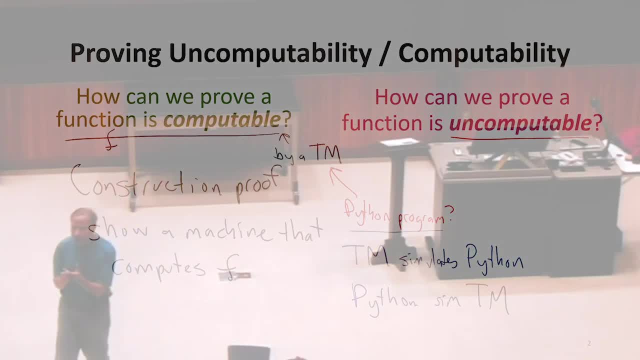 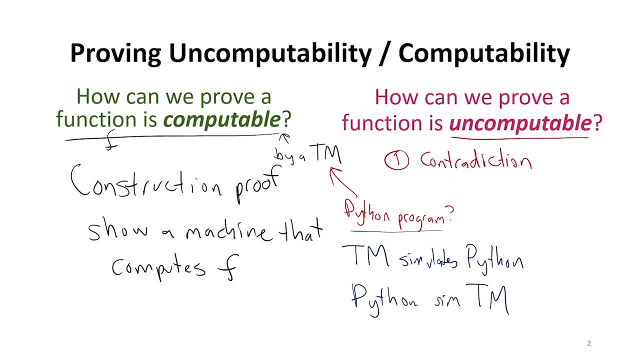 what do we have to do? Yeah, So we have two main strategies. One is contradiction: We're showing that if we could compute this, something impossible would result. The other main strategy is- it's also kind of contradiction proof to say: here's something we know is uncomputable, that we could build if we had this. This is a 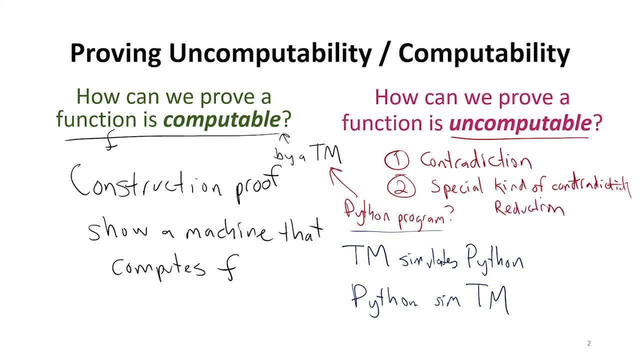 special kind of contradiction. So we have to do a reduction that shows some problem that we already know is uncomputable. Any problem that you already know is uncomputable can be used for this. Let's try an example. Is addition computable? What would your intuition tell you? 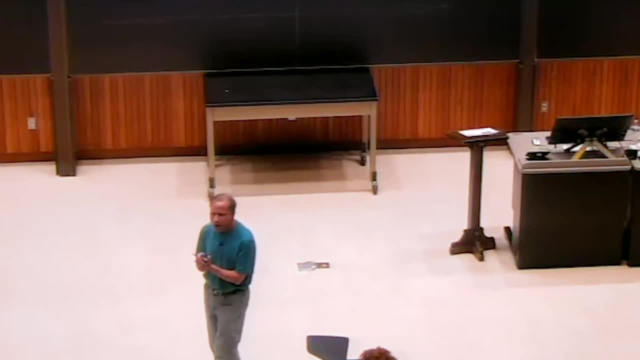 It would tell you: probably yes. The other thing it should tell you is: well, define addition. We can't answer a question like: well, is addition computable? We can't answer a question like: well, is addition computable? We can't answer a question like: well, 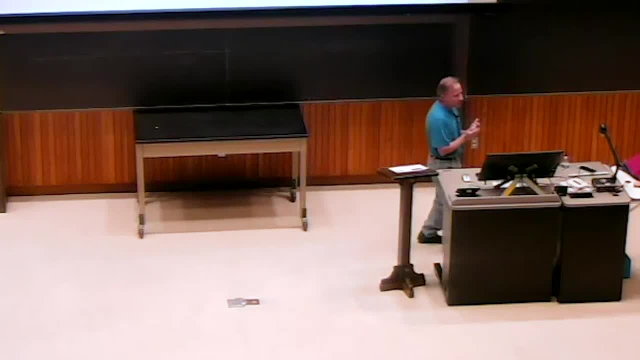 is addition computable? We can't answer a question like well, does addition exist? No, So we can't answer the question about whether something's computable or not, unless it's defined in some precise way. So we better define addition. How should we define? 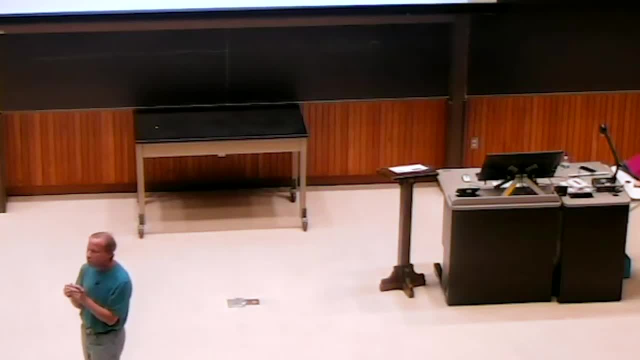 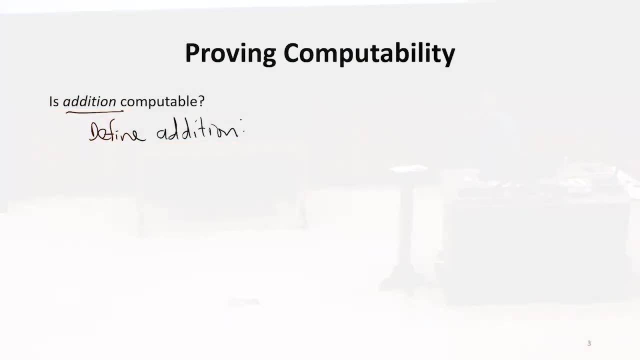 addition. How do we define a function? Yeah Good, So let's assume we've got a mathematical, we've got the mathematical definition of addition already. Let's assume we have plus defined on the naturals. We know plus is a function that takes two naturals in and it outputs a natural And 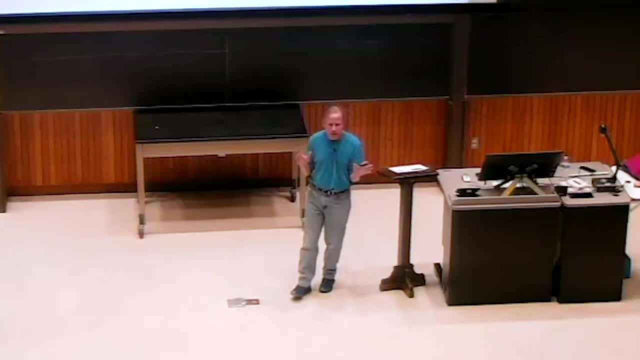 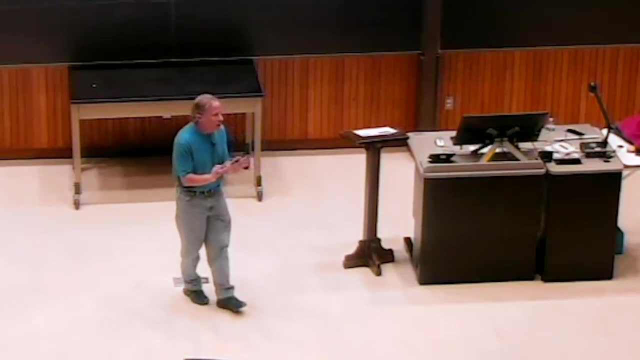 that function is defined and we have a good notion of what addition means. If we're asking, is it computable by a Turing machine, we've got to define it as a function that makes sense to a Turing machine. So we've got to say what the 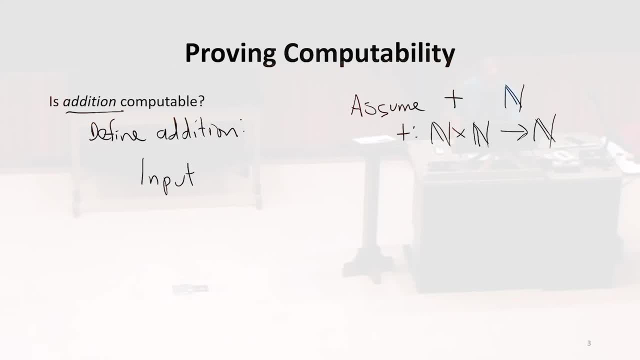 input is: What is the input to a Turing machine? Is it two natural numbers? It's got to be something that we can encode on a tape with a finite sequence of symbols. So we've got to describe the input and the input. if we're being 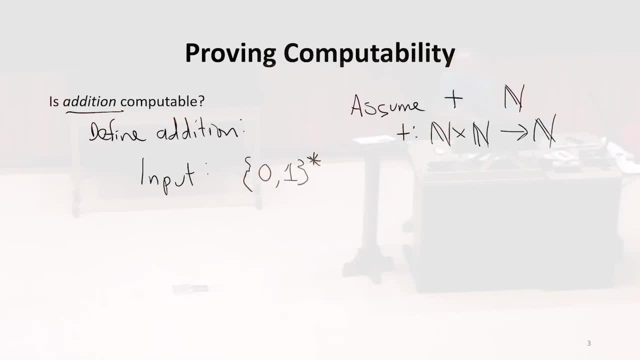 careful right. So the input is some string of zeros and ones, or maybe we could add some other symbols to our alphabet. Maybe it's going to be useful if we add a plus symbol And let's say it's of the form, the sequence we've got. 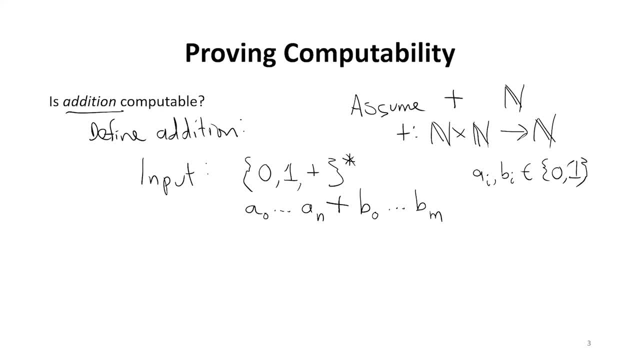 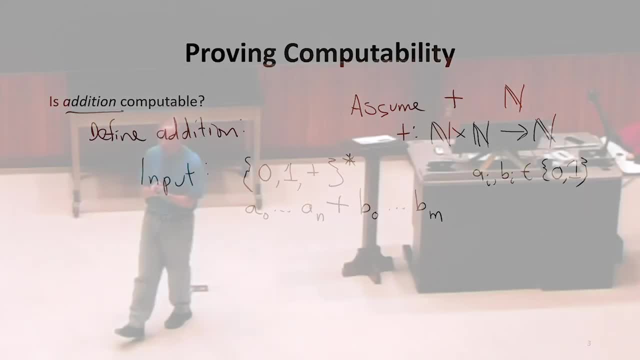 all the little a's and little b's are zeros or ones, and we're using our special plus symbol to separate them. Okay, so that's our input, And now we've got to say what the output should be. So how do we know what the output should be? 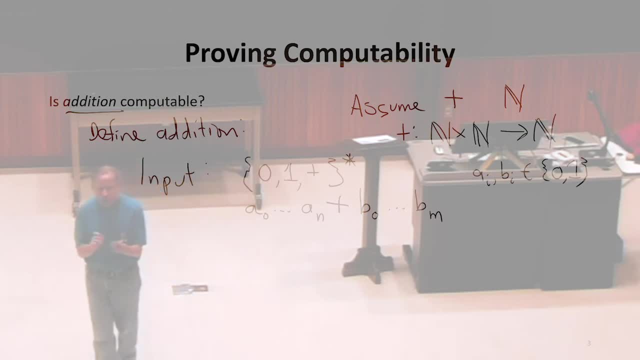 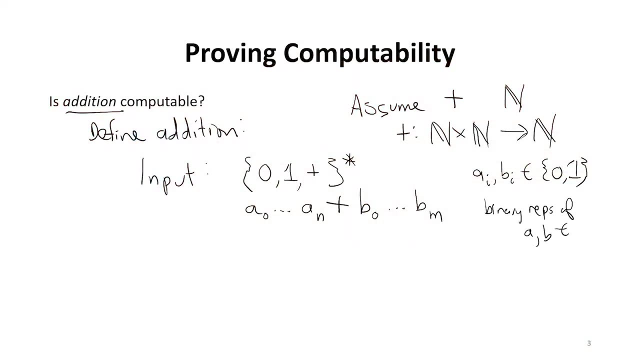 How will we define the output? Well, we want at the end of the machine execution the tape is going to contain. and now we're going to say, like these are binary representations of naturals, and then the output is going to be the binary. 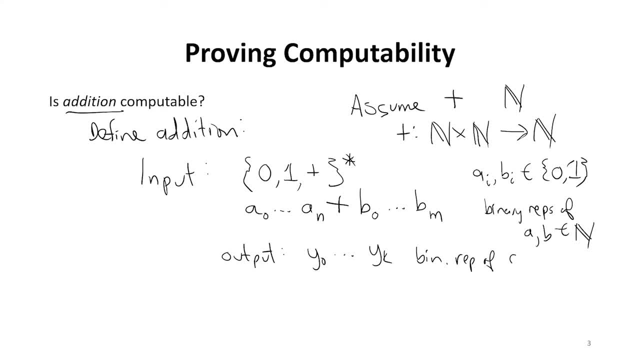 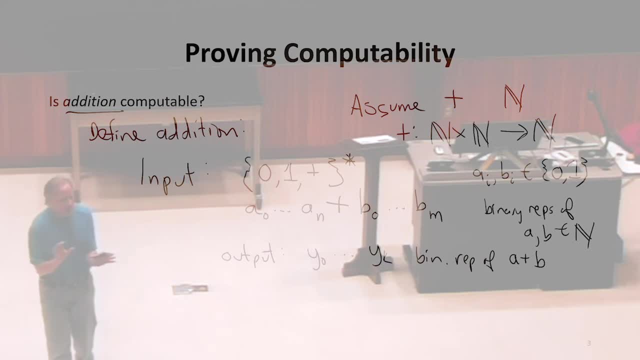 representation a plus b, where that plus is the natural number plus. So if we want to ask a question whether something's computable by a Turing machine, we've got to define a problem, We've got to define the inputs and what the required. 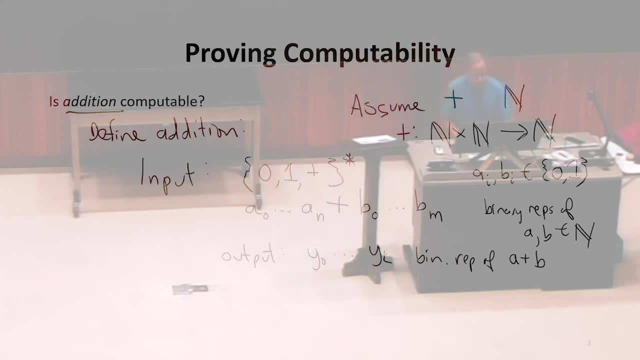 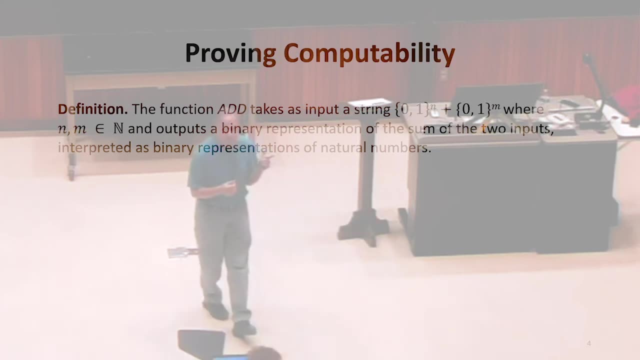 property of the output should have. Now we've got that definition, how do we prove it's computable? Yeah, So certainly this is one where it would be nice to have a Python program rather than a Turing machine, But it should also raise the little questions. 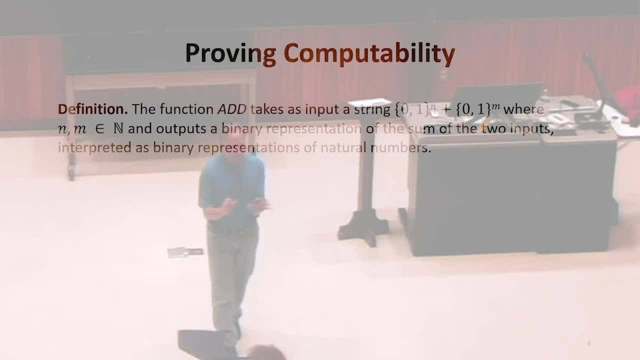 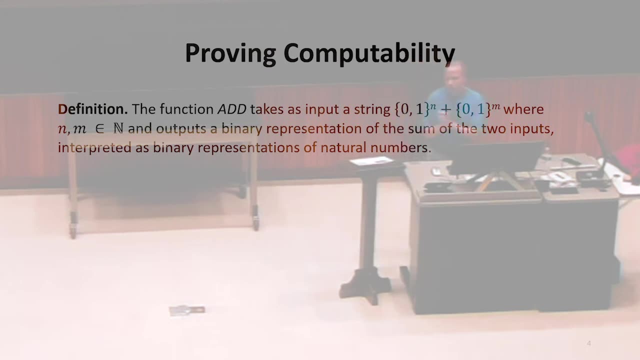 of how. if we built our Turing machine to simulate Python, it would need to include a way to simulate what plus does in Python. We're sort of offloading all the complexity of this to assuming this Turing machine that implements Python exists and we haven't. 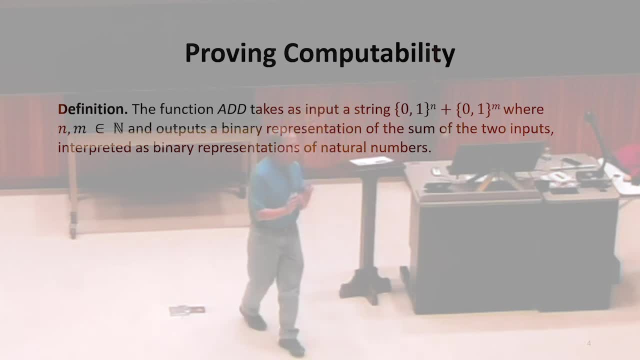 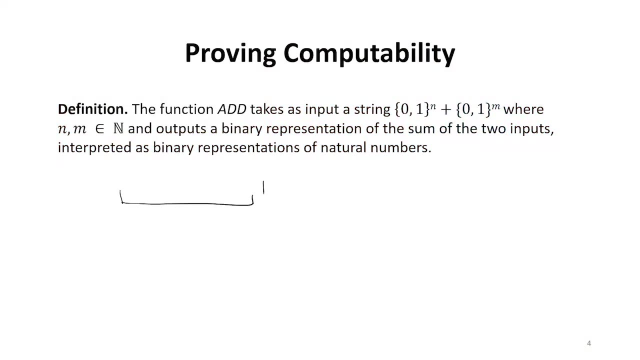 actually done that. If we didn't want to do that, we'd have to get some sort of intuition of: well, if we're going to do add as a Turing machine, we're going to start with this as the input. Writing a full Turing machine like this would probably take longer than you have for the 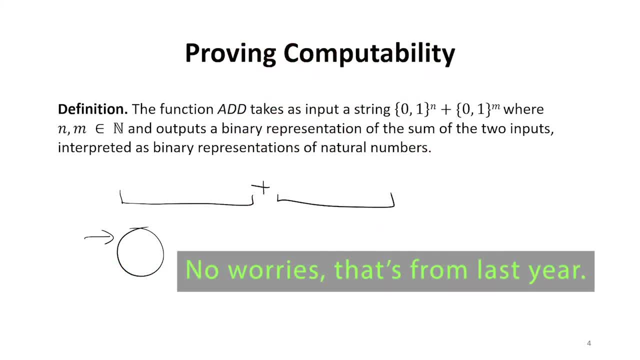 exam and is not that interesting, but you should have a sense that you could do it. Well, you've got to probably look for the number before the plus, so you're going to have something that's going to move right without changing it until you see the plus. 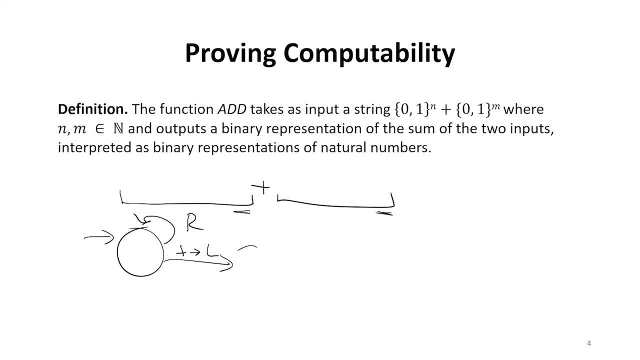 and then you're going to move left and then, based on the plus, you're going to have something that's going to move right without changing it until you see the plus, and then, based on whether that's a 0 or a 1,.